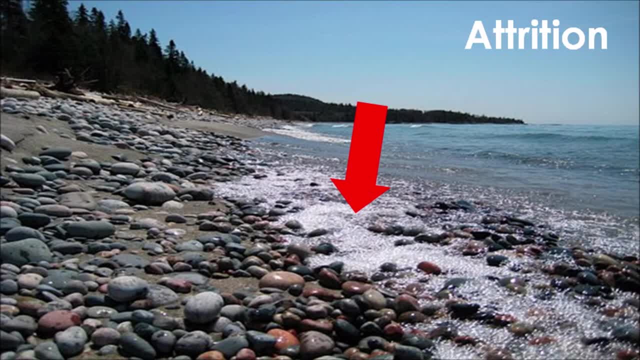 into smaller fragments. This is why you will often see pebbles or shingle located along your shoreline where their edges have been rounded off, because abrasion is this constant smashing together of these particles and they create these lovely rounded edges as they bash together, or even 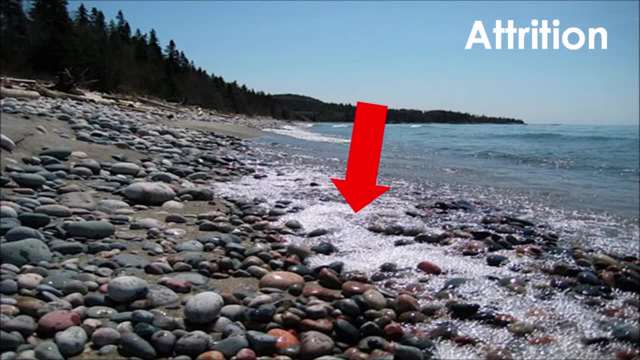 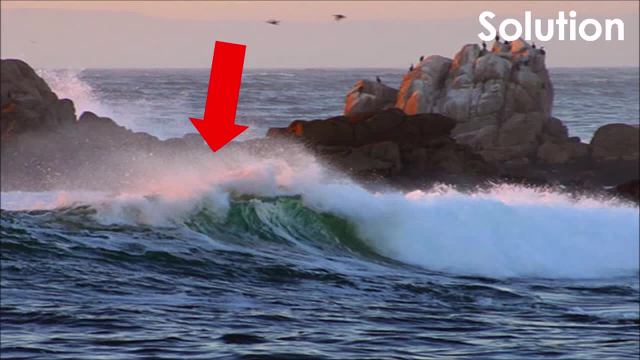 sometimes rub together within the water And finally we have solution. Solution involves weak carbonic acid that is present within our seawater and that will dissolve rock, specifically chalk and limestone rock, and it will eventually slowly wear away the cliff faces and any material made of chalk and 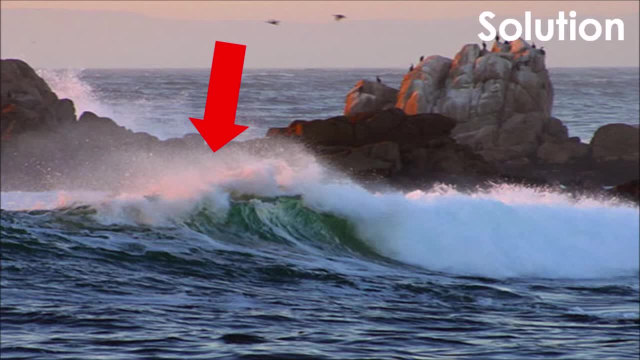 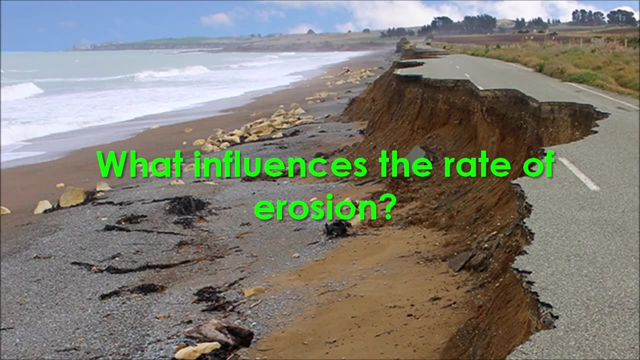 limestone by this weak carbonic acid in the seawater, dissolving the particles F's & Qs particles. So if we then consider what influences the rate of erosion, because every single coastline in the world will potentially have erosion taking place along it. However, some coastlines are 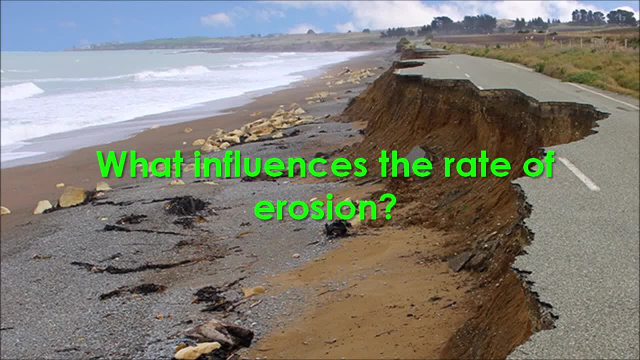 eroded much faster than others, which unfortunately means that some coastlines are at risk of retreating and moving back, whereas other coastlines experience very little erosion. So the first thing to influence the rate of erosion is something known as fetch, And we have 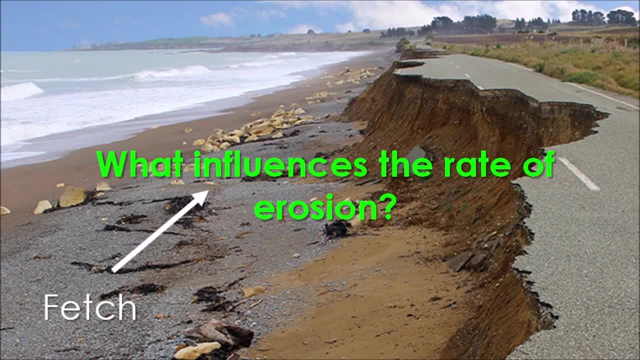 covered fetch in a previous video when we looked at the importance of waves. When we're talking about fetch, we're talking about the distance over which the wind has blown, So the greater the fetch means that the energy that has been created from the wind creating friction over the surface of 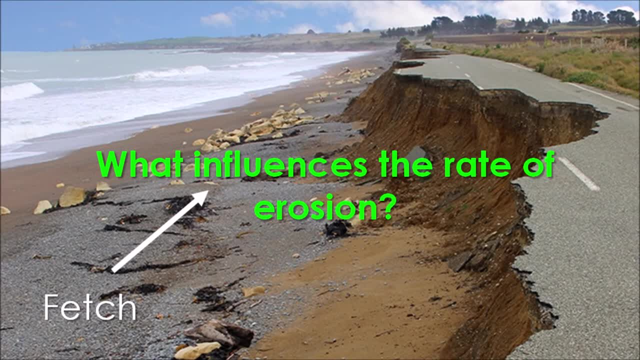 the waves has increased because of the length of time over which the wind has blown, as well as the distance the wind has traveled from. We've, then got strong winds. So, again, the strength of the winds will determine the rate of erosion, whether erosion is taking place fast or slow on our 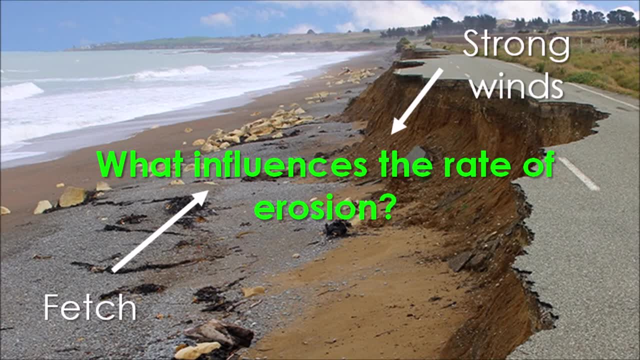 coastline, So strong winds blow for a very long period of time and they are known for creating destructive waves. Again in a previous video- the importance of waves- I'll put the link in the description box below- we looked at this idea that destructive waves have a very weak swash, but a